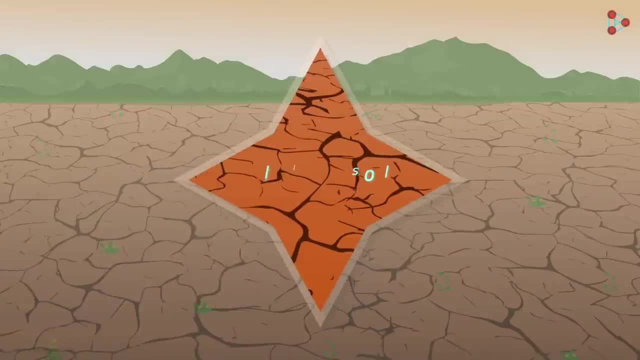 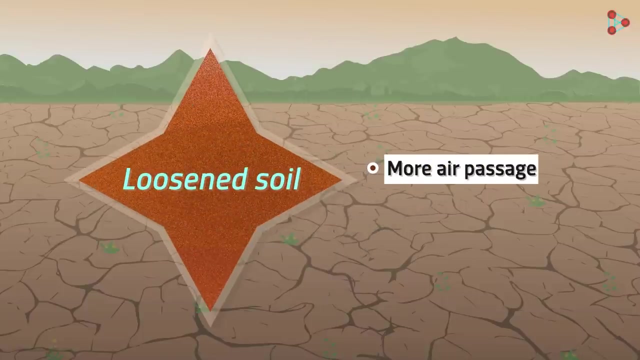 production. Yes, soil is usually found solidified into hard chunks of soil mass. This soil needs to be softened and loosened. Why does soil need to be loosened up before cultivation? The answer is simple: Loose soil will allow more air to pass to the roots of the plants. This will, in turn, aid 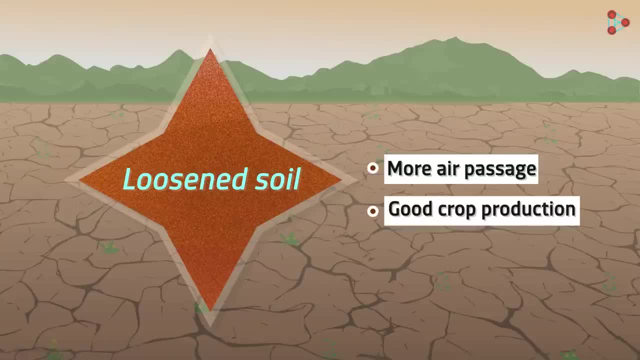 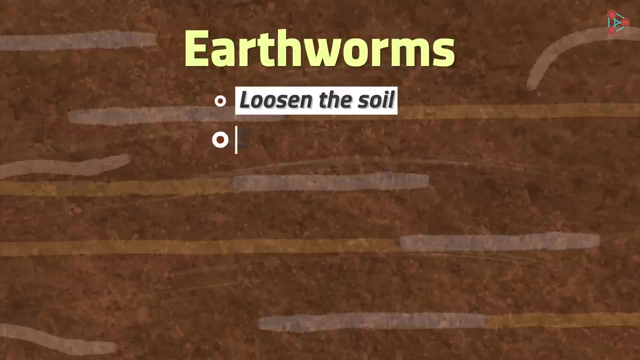 the growth of the plant, leading to good crop production. Do you know any natural agents that help this process? We usually refer to them as friends of the farmers. Yes, the answer is earthworms. They help loosen the soil and also in soil aeration. Do you know another advantage of loosening of the soil? 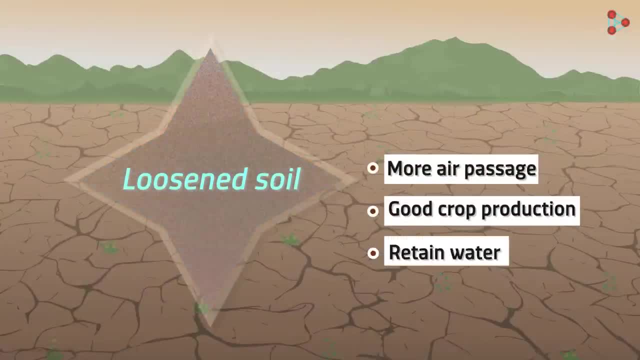 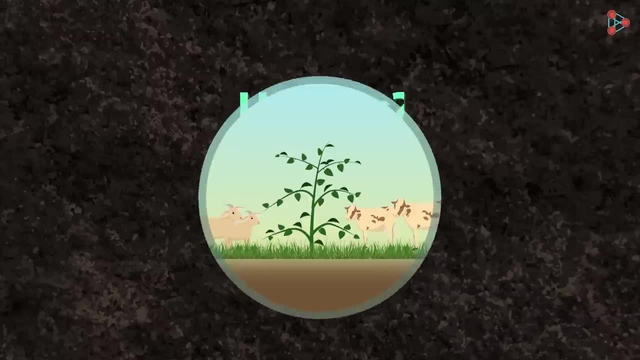 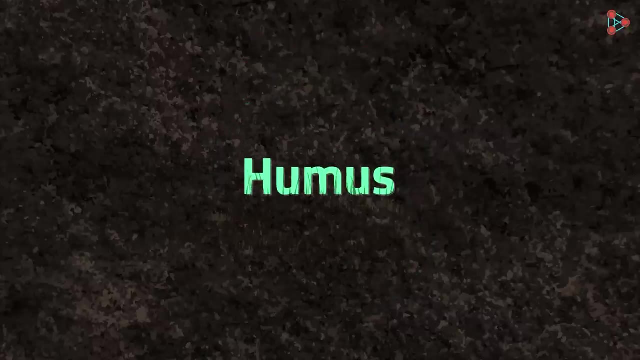 It also helps the soil to retain water. It then leads to the growth of favourable microbes that help to produce humus in the soil. What exactly is humus? As we know, all living things die. their remains are decomposed And nutrients are returned back to the soil. The microbes help in this process of decomposition. 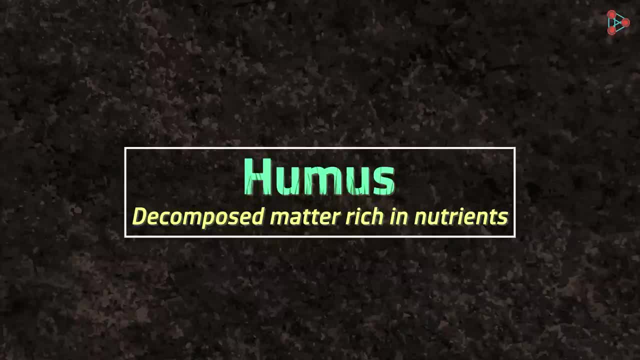 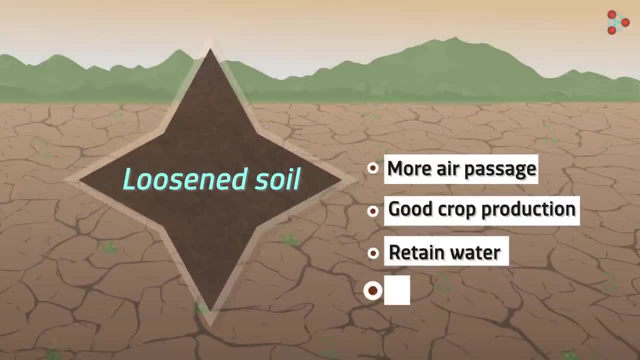 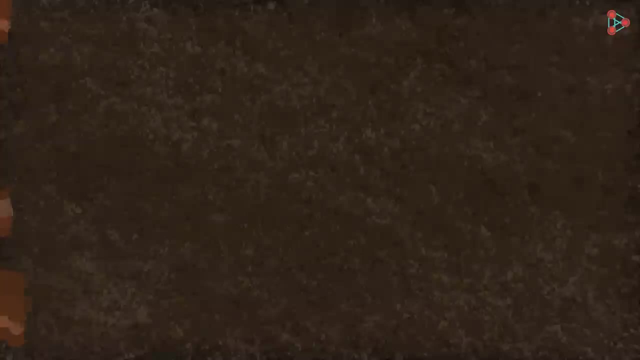 This decomposed matter is rich in nutrients and is known as humus. It is what plants depend on for nutrition. Do you also know that loosening up of soil has yet another benefit? Plants mostly take nutrients from the top layers of soil and they are unable to go deeper into the soil. 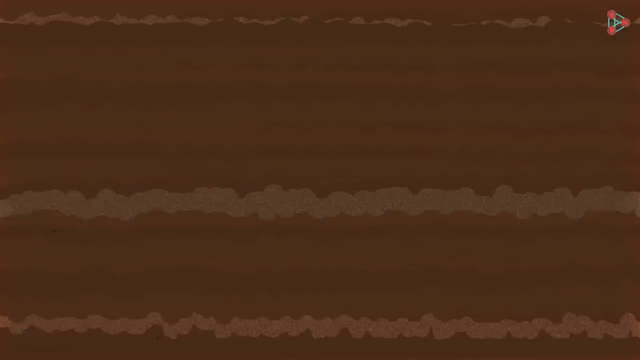 Loosening up the soil helps to turn the lower soil and makes it accessible to the environment. It also helps the soil to retain water. Do you know any natural agents that help this process? Yes, the answer is yes. All natural agents are brought to the soil, the roots of which are the easily accessible. 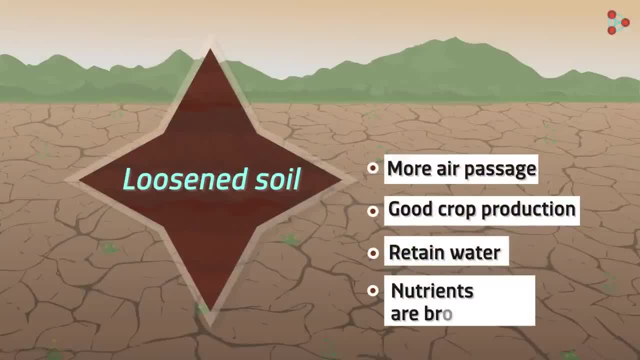 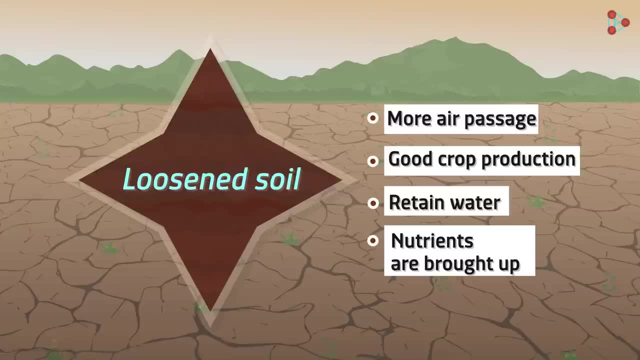 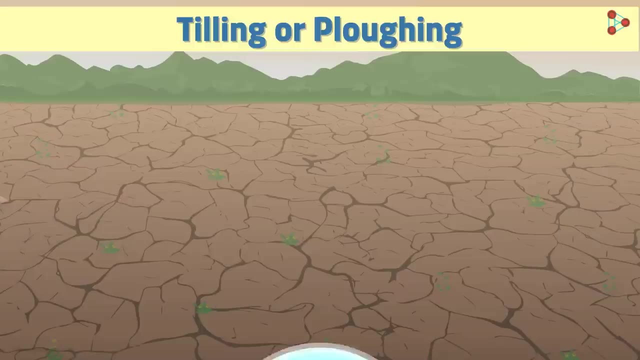 to the plant. Thus the nutrients in the lower layers are brought up to the upper layers of the soil. So what is this process of loosening and turning of soil called? We call it tilling or ploughing in agriculture. How is tilling and ploughing done by man? Have you heard of an equipment? 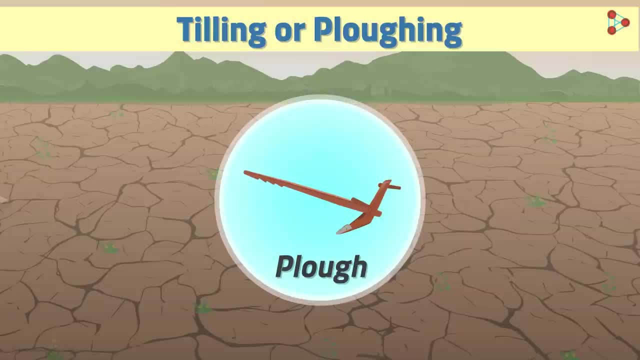 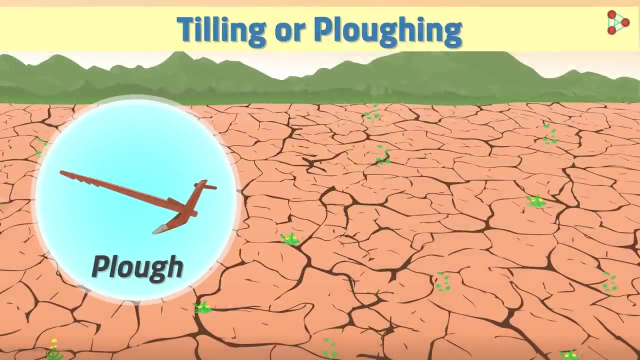 called plough. Yes, I am sure you have. It helps to loosen the soil. But what if the soil is hard? Would it be easy to plough? No, it won't be. Hence the soil may have to be watered before ploughing. 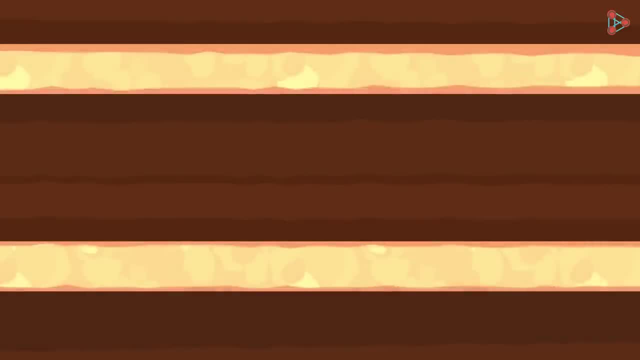 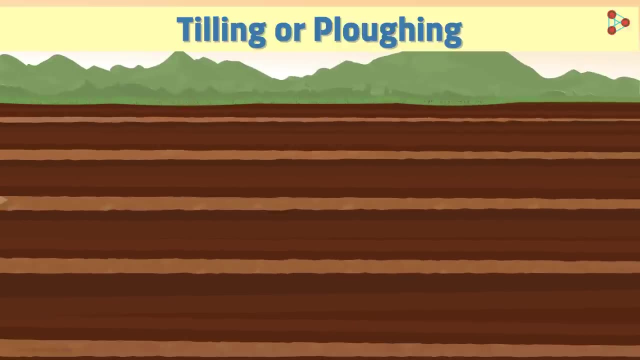 Even after ploughing, huge chunks of soil could be left behind. These chunks need to be broken down into smaller fragments. Soil also needs to be levelled so that the land is even and sowing of seeds can take place on this land.